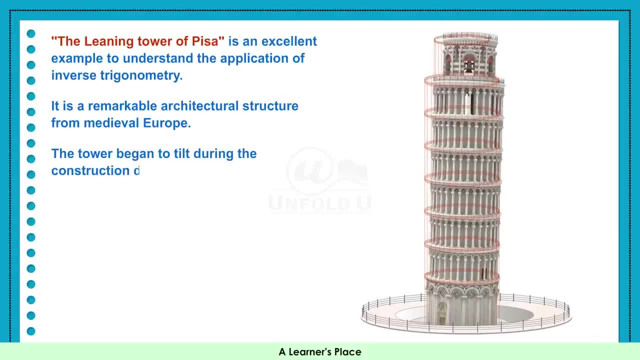 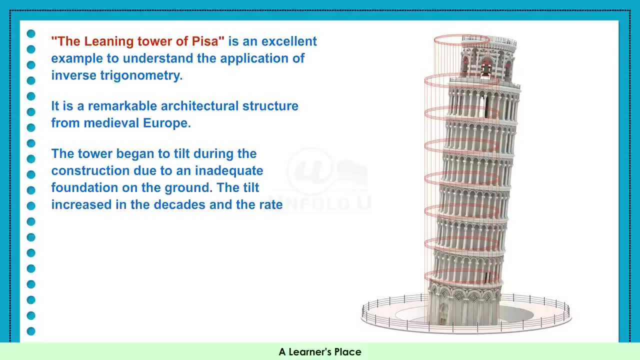 We normally see it it documentary on aкретik Drive from one side construction due to an inadequate foundation on the ground. The tilt increased in the decades and the rate at which the tower started to lean was such that it would have fallen with time. 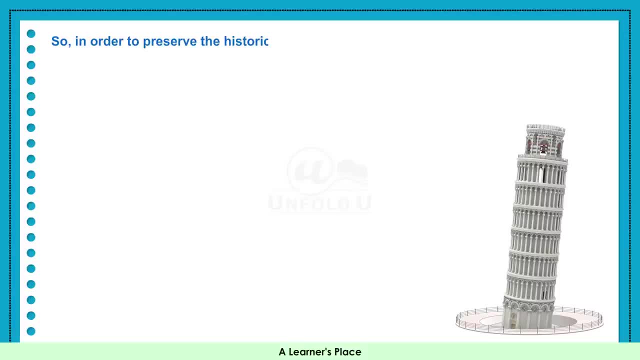 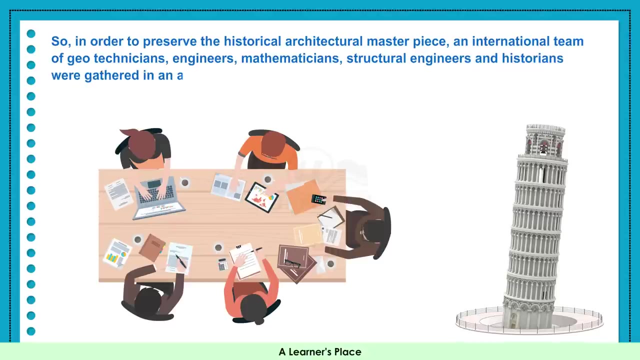 So, in order to preserve the historical architectural masterpiece, an international team of geotechnicians –, engineers, mathematicians, structural engineers and historians – were gathered in an attempt to save the famous landmark. For this, first of all, the angle at which the tower was leaning was calculated. 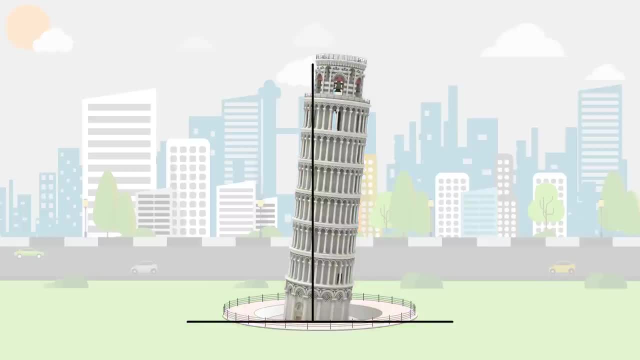 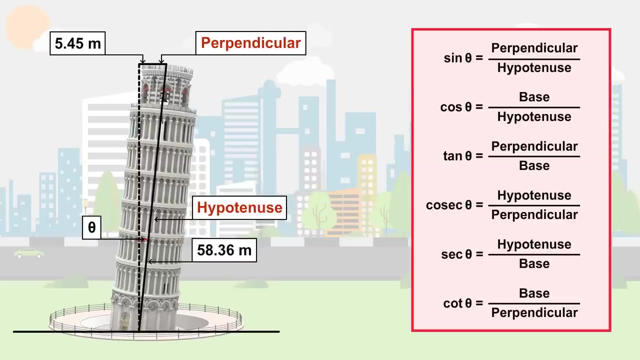 From the figure we can see that the height of the tower acts as a hypotenuse and it is distance from the centre acts as the perpendicular. So they had the value of perpendicular and hypotenuse. From the table of trigonometric ratios it is clear that sine theta is equal to perpendicular. 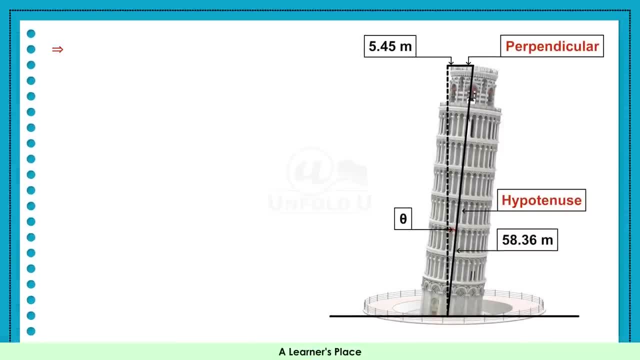 upon hypotenuse, which implies sine theta is equal to 5.45 upon hypotenuse. So theta is equal to 5.34 upon 58.36,, which implies sine theta is equal to 0.09338,, which implies theta is equal to sine inverse of 0.09338,, which implies theta is equal to 5.3580. 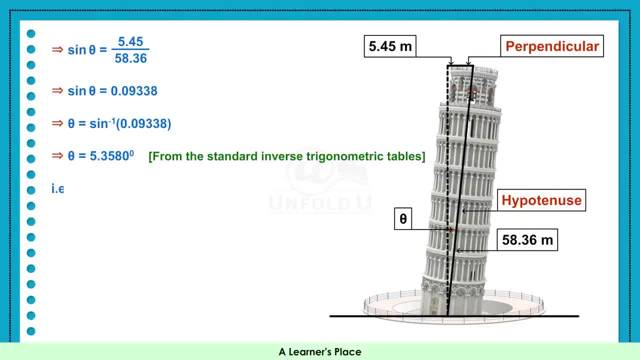 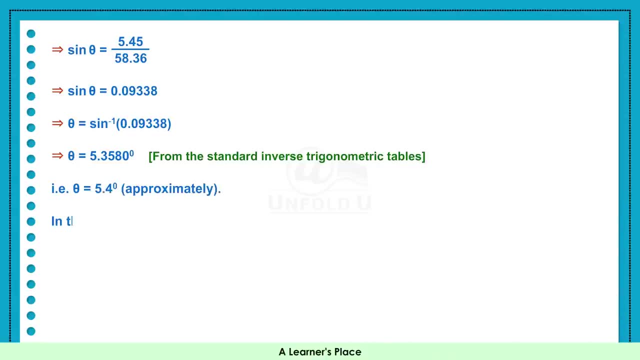 degrees, That is 0.05.. So in this way, theta is equal to 0.03338.. is theta is approximately equal to 5.4 degrees. In this way, they used the concept of inverse trigonometry to find the angle at which the tower was leaning. Therefore, the tower had 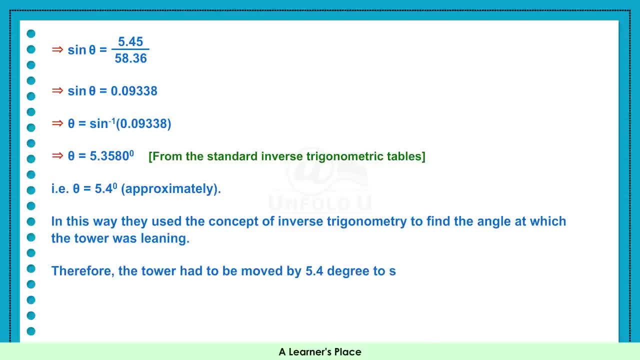 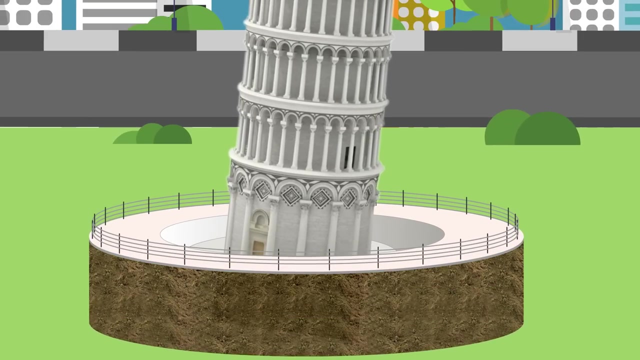 to be moved by 5.4 degrees to straighten it, But the government of the city considered it very important to retain the tilt of the tower, due to the role that this element played in promoting the tourism industry of Pisa. So it was decided that the tower should be. 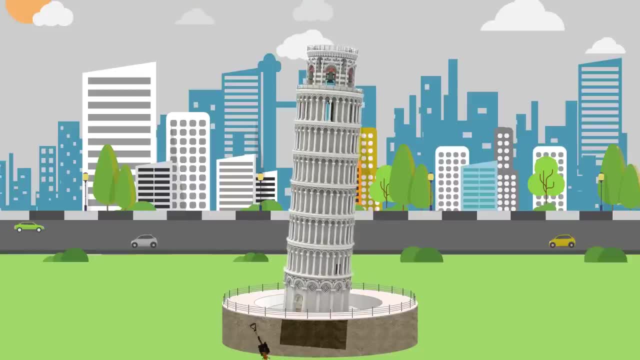 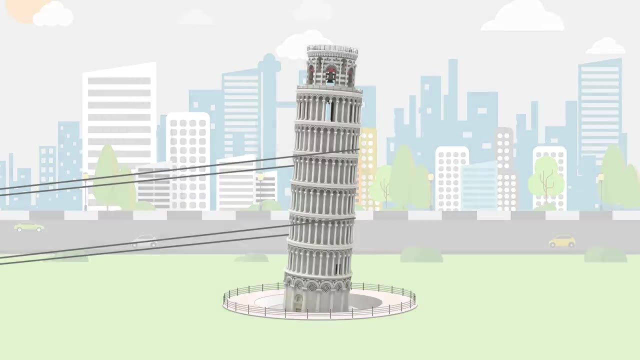 moved a little and the foundations were reinforced and the tower itself was encircled with steel cables, Due to which tower was moved by approximately 1.55 metres. As a result, the top of the tower was displaced horizontally from the centre and the height. reduced to 56.67 metres. From the figure we can see that the height of the tower is as high as 2 feet. Those seus can be casually measured. cut in length, However, the size of the tower can be adjusted in several ways, from 0.65 to L in some situations. 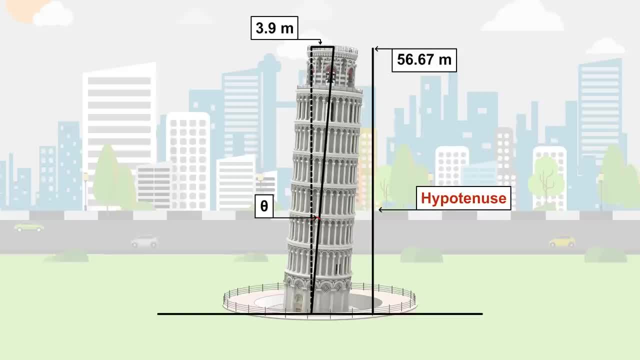 After the averagation was made, the pitch of the soil was stretched towards a jointage. power acts as a hypotenuse and its distance from the centre acts as the perpendicular. So again they made calculations with new values of perpendicular and hypotenuse. 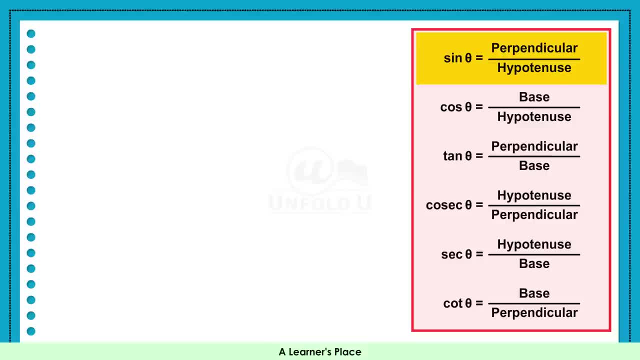 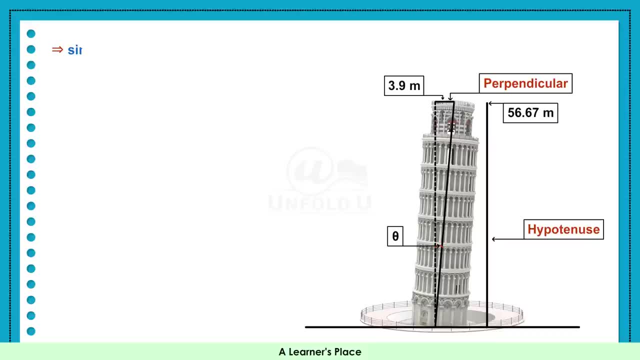 From the table of trigonometric ratios: sine theta is equal to perpendicular upon hypotenuse, which implies sine theta is equal to 3.9 upon 56.67,, which implies sine theta is equal to 0.0688,, which implies theta is equal to sine inverse of 0.0688, which implies theta. 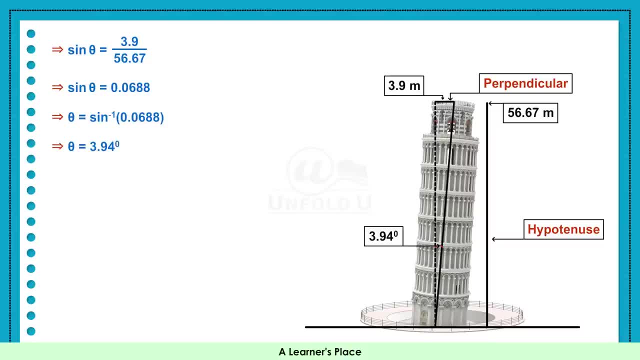 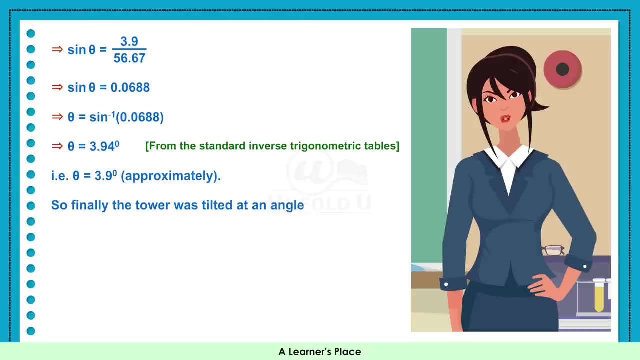 is equal to 3.94 upon 56.67.. That is, theta is approximately equal to 3.9 degrees. So, finally, the tower was tilted at an angle of 3.9 degrees and declared safe for the next 300 years. 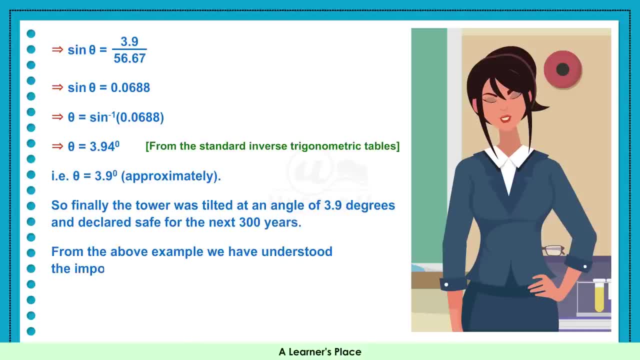 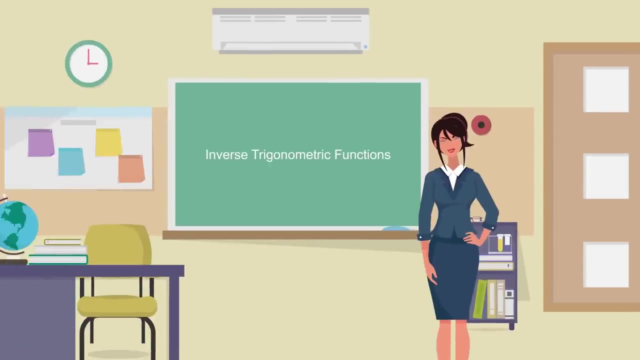 From the above example, we have understood the importance of mathematics in our daily lives. Moving towards the next step, you should also try to visualize things in real life from mathematical point of view, which will make learning easier and interesting. Thank you, We will meet again in the next session and discuss some other topics and try to connect. 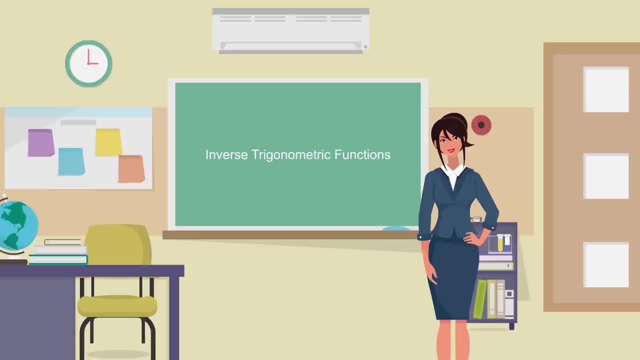 them with practical examples. Thank you,